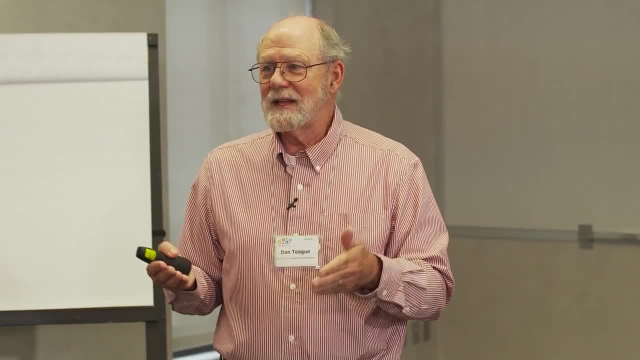 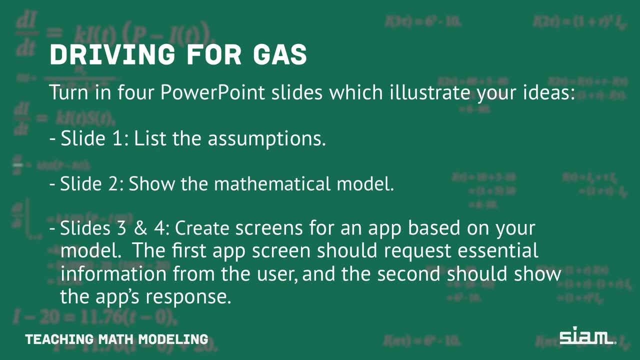 to make an app for their smartphone that someone could use to answer this question. What are the assumptions you're making that go into your model? That's one slide. What is your mathematical model? What have you computed That's going to be used by the cell phone And what is the presentation they have where? 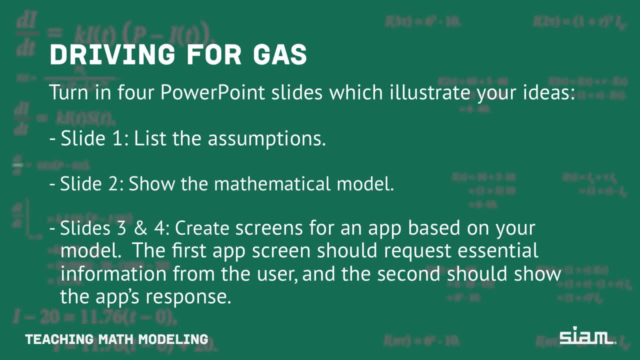 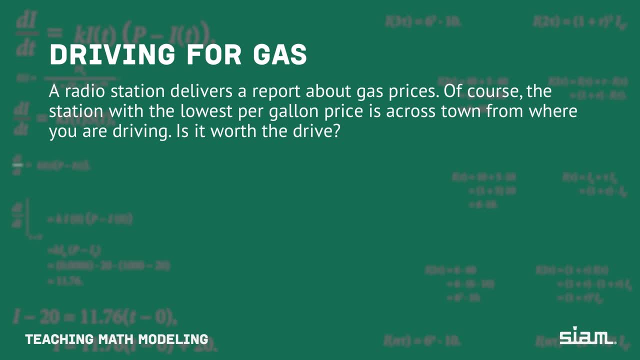 they put in the information, What information do you ask from them And what information do you give back to them? So we're going to be looking at just the basic part of the problem. Given this question of when should you drive off your path for gas, what I'd like to do, 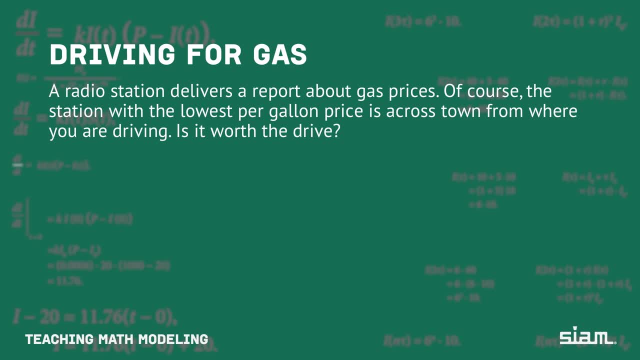 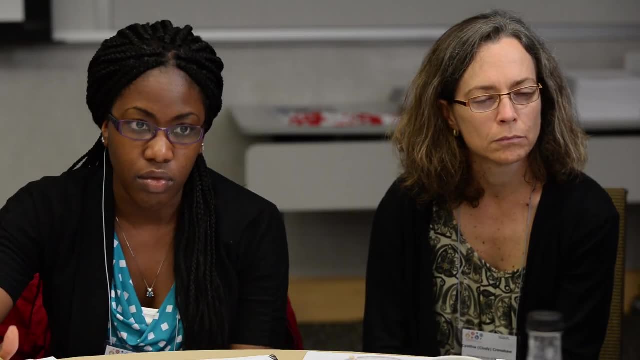 is just put on the table. what are the important considerations that you're going to have to consider? What are the things that you've come up with? Miles per gallon of the car that you're driving, so that information needs to be known. 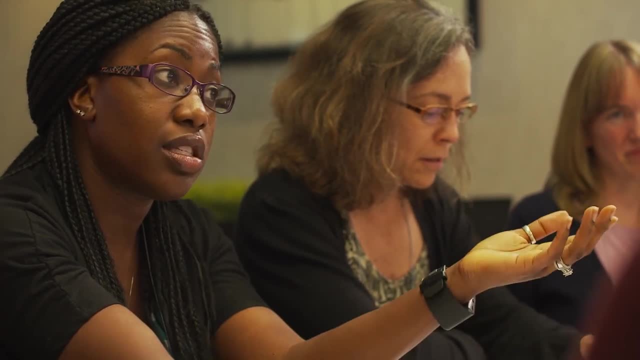 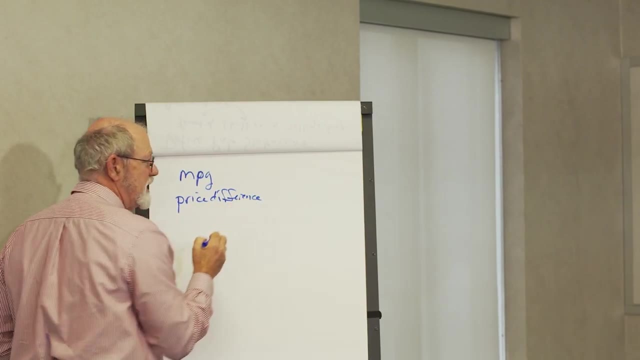 You mean, like it's two cents difference, I'm not going to waste it, it's 50 cents, I might actually make some money. So the difference in gas prices and the difference in time, Is that different from knowing the two prices? Would you rather know the two prices or just? the price difference. You're using some of the gas that you guys bought. You're using gas to get back from that station right, So that's not really usable gas. The fundamental question is how far away, yeah, how far- is the station that's not proximate. 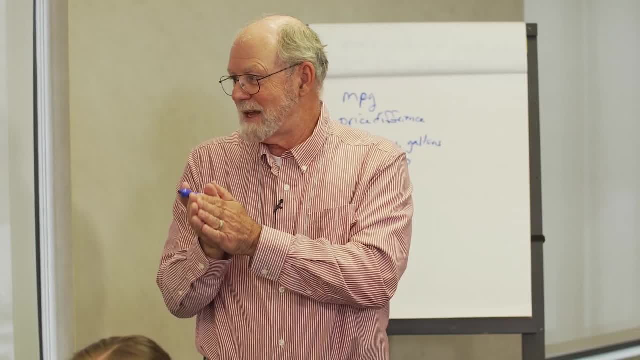 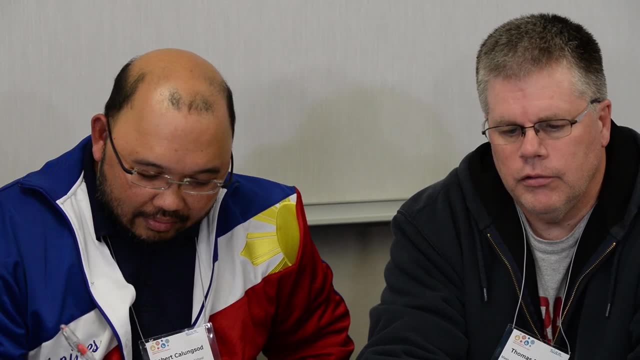 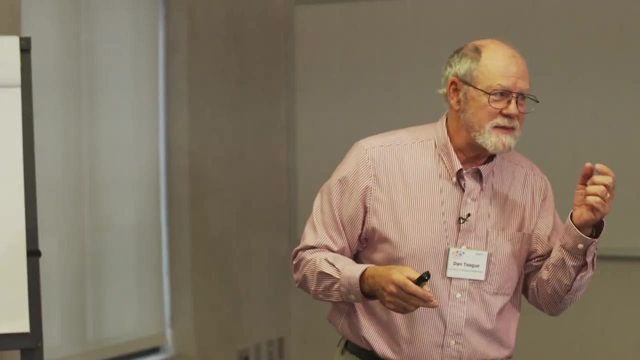 to your path, And the result of that is you've got to use gas to get there. One of the things that I ask the students to do is to try to again just as before. a particular example of this problem, And one way of thinking about this, is to ask them. 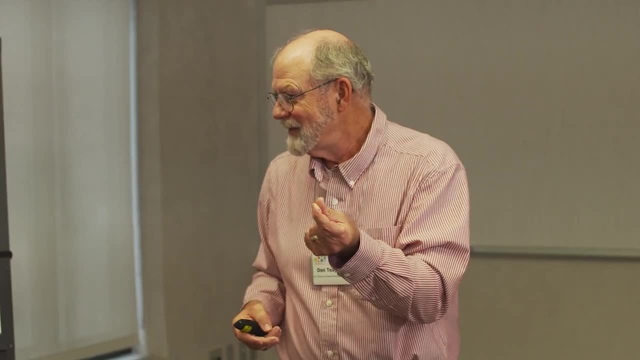 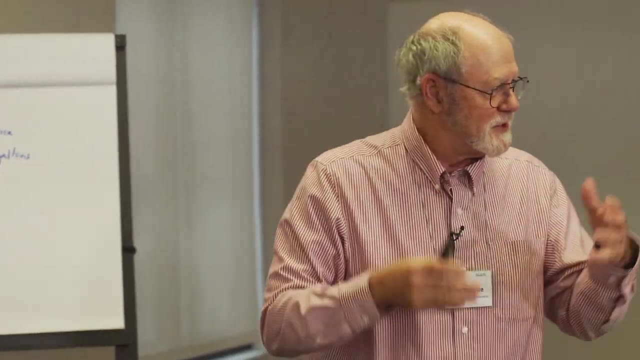 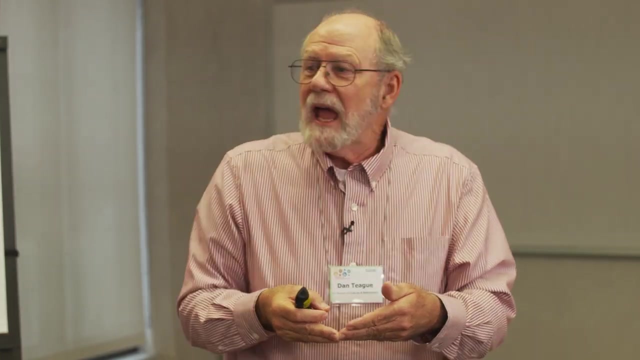 suppose your teacher had given you a word problem. based on this idea, Could you create the kind of just standard word problem that he or she would give you And solve that? Just turn it into something that they're comfortable with, Turn it into a specific. 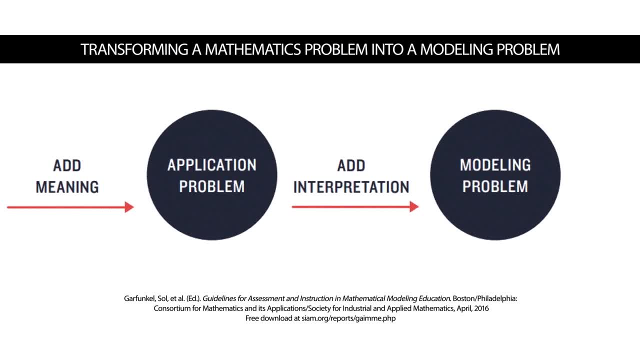 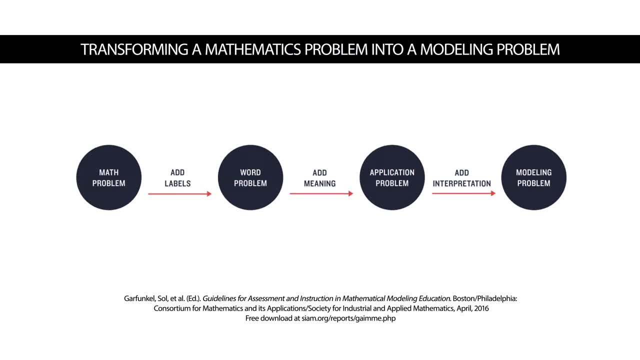 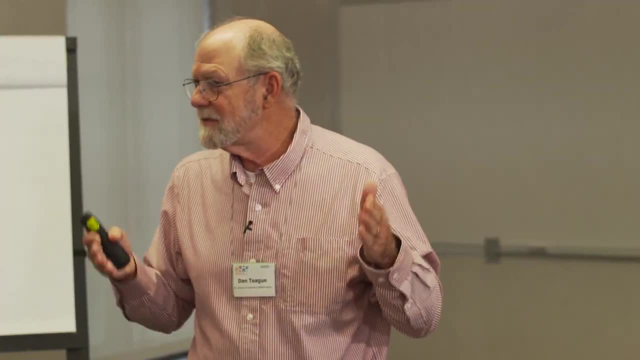 example of the general problem So you might want to think about. can you draw a diagram of the problem you're trying to solve? We always want to start. have them start with the simplest version of the problem that contains the essence of the problem. Try to strip away. 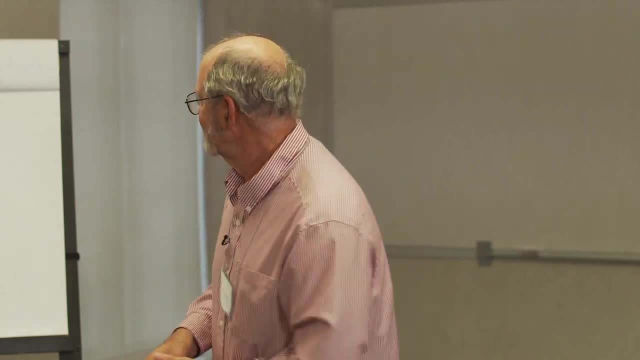 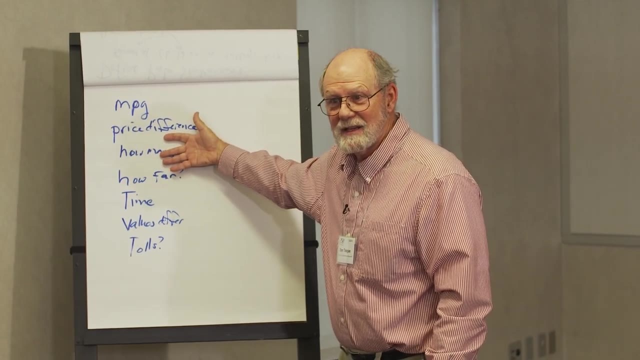 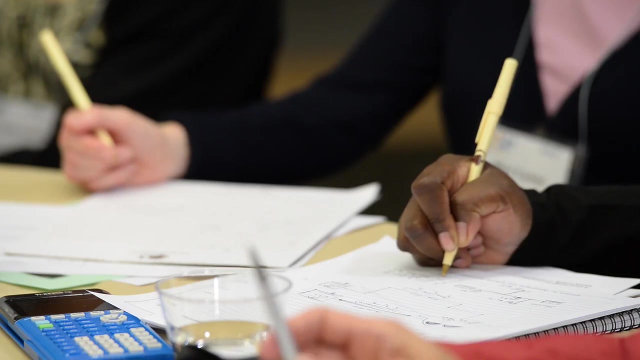 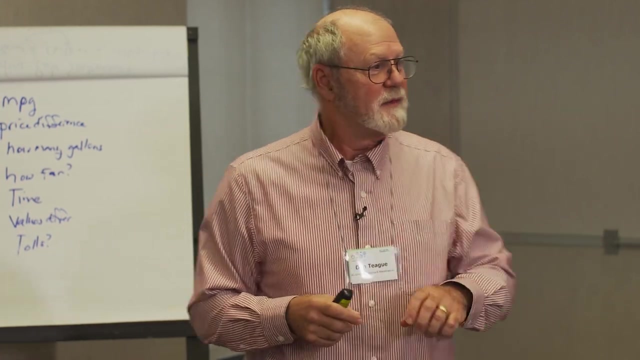 as much stuff as you can, but still contains the features that each of these still has some meaning and effect on the problem. So take a minute and draw a picture of the problem you're trying to solve. Again, think about your students. they'll draw lots of different things. There are a. 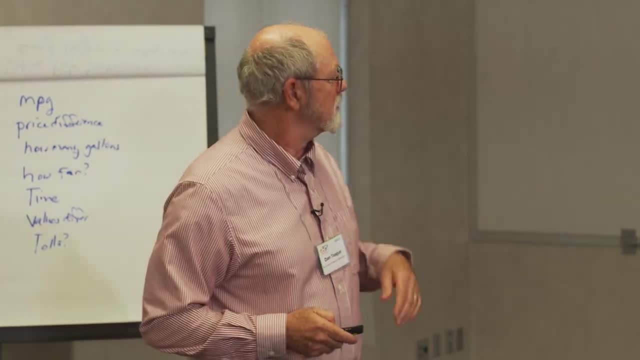 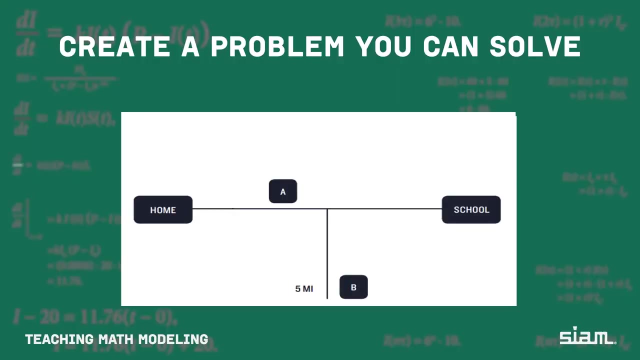 lot of sort of triangles. One of the things I try to get again get them to do is to draw something simple, to try and make it as simple as possible. For example, something like this: going from home to school, school to home, home to school, school to home, There is a 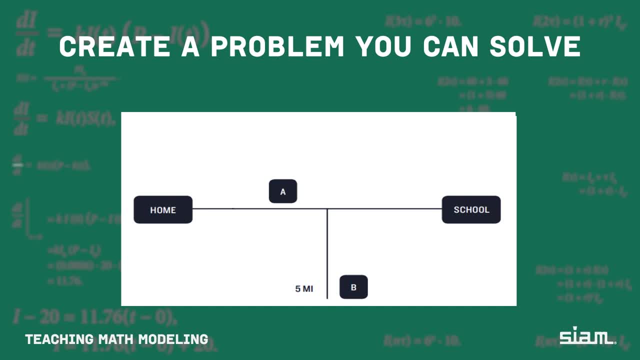 gas station A. that's on the route so it doesn't cost me anything at all to get there. There's a gas station B that's off the route. I've got to get to the gas station and get back to my route and then continue. Once I solve the simplest version of the model, then I 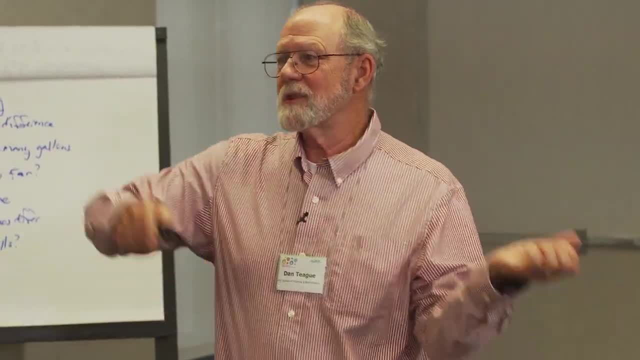 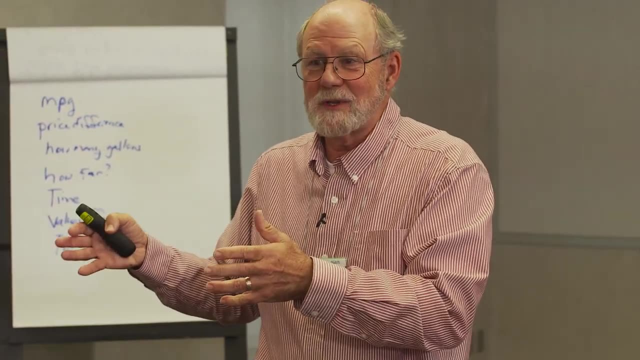 want to make it more realistic, But I don't want to start with the more realistic problem to begin with, because it may in fact be too realistic and I struggle with solving it. If I can't solve the simplest version, I'm not going to solve the more complicated version. 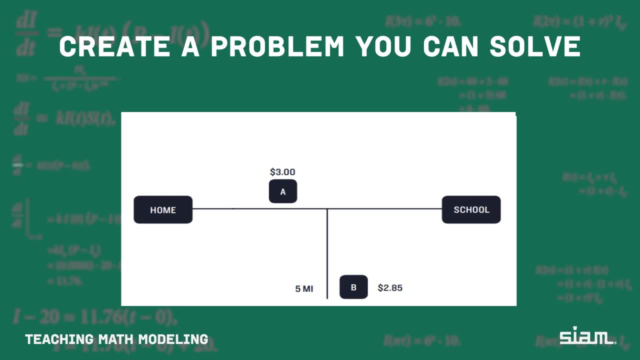 But, more fundamentally, the insight that I get by solving the simplest version is often times very, very easy. The harder problem is just a modification of that earlier solution. The whole idea of the modeling cycle is to get a solution. that solution becomes new. 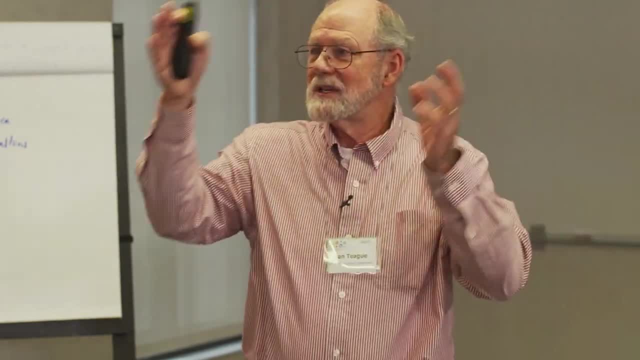 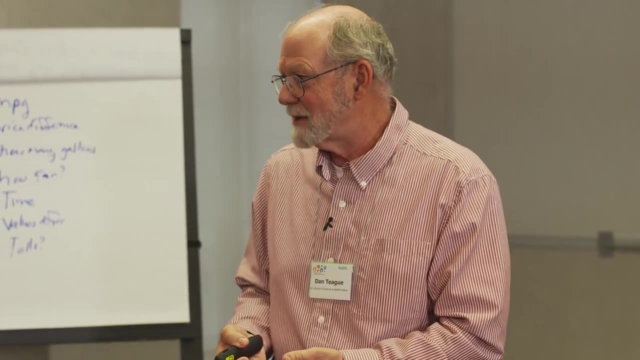 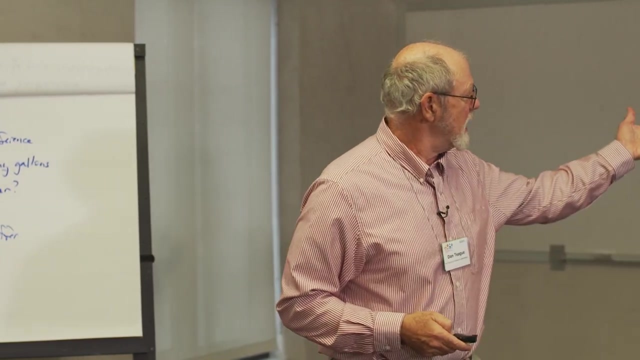 information, you start from a different place than you did originally and you keep adding in reality as you go through, rather than trying to create a fully realistic model initially. That's one of the things students struggle with and you have to really work with them on. So I 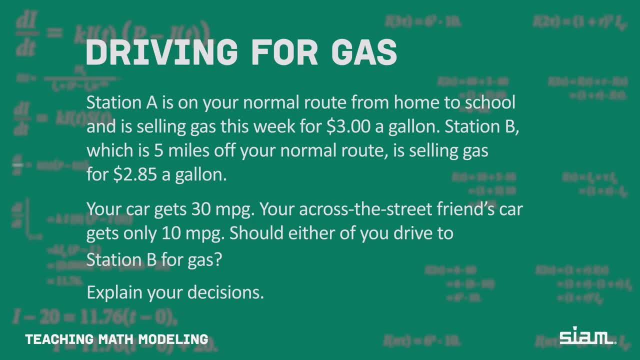 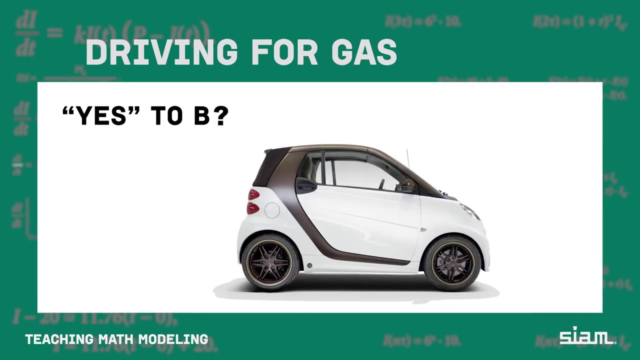 draw a picture of it and then I just turn it into the problem. my teacher would give me Simple numbers: 5 miles, $3.00, $2.85 a gallon. Can I solve this problem? Can I create a car where the answer is yes, I would go to B. Could I create a car where the answer would: